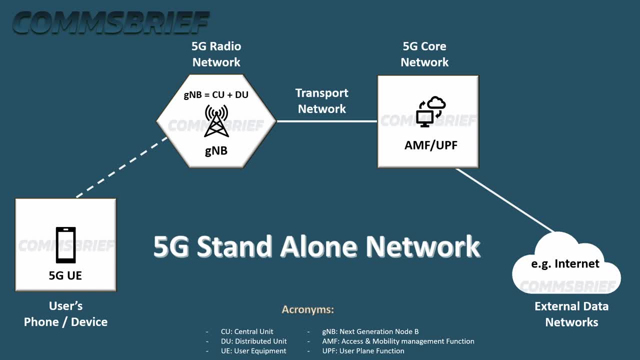 The 5G core network consists of several nodes which we will look at in the next slide. Generally, the key nodes representing the 5G core networks in most documentation are AMF and UPF. UPF is user plane function, AMF is the access and 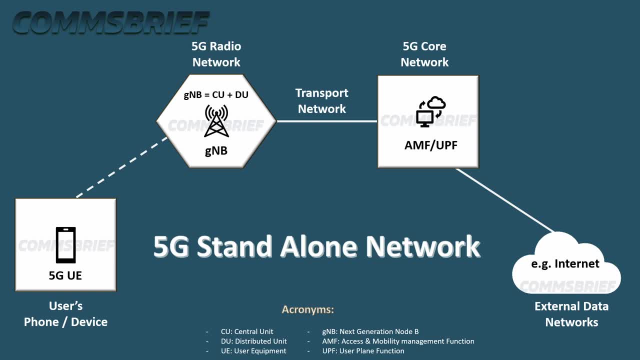 mobility management function. Let's now look the nodes and functions that 5G core groups fly within at these five Switch через 5G egress一個 demonetization nodes called Pol-whole Interface UAV. the Functions that do these functions are the following for each node: 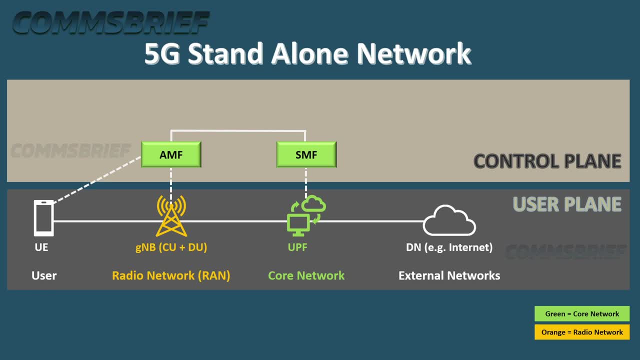 A cool small list of nodes for all: Page cleans and folders, PQ, wells, DLF, submission tudo, such as CDN, colaborated tough stats and Greed or splitting data in paths, Transaction and routing. forideo people мышsah at the nodes and functions that 5G networks use. The network architecture can be seen at at least. 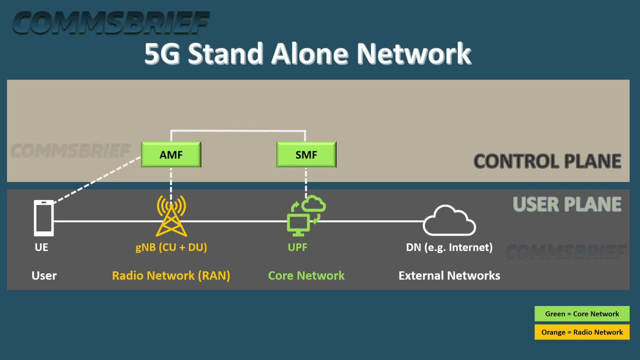 two levels: the user and control planes. The control plane carries control functions, such as signaling traffic, and the user plane carries user data, for example, the content of the YouTube video you may be watching on your phone. A mobile phone is connected to the base station GNB. 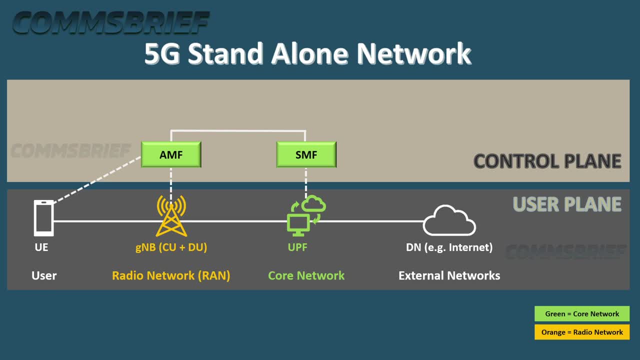 linked to AMF and UPF in the core network UPF user plane function which, as the name suggests, is part of the user plane and connects a mobile phone via GNodeB to outside networks like the internet. UPF is connected to the session management function SMF in the control plane. 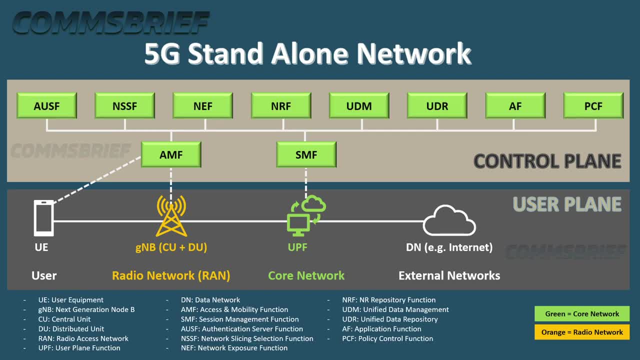 UPF oversees service quality and applies policies that the PCF policy control function sends via SMF. There can be more than one UPF and, for low-latency communication, local UPF can be used to avoid transmission delays due to long distances. Let's now talk about SMF, or session management. 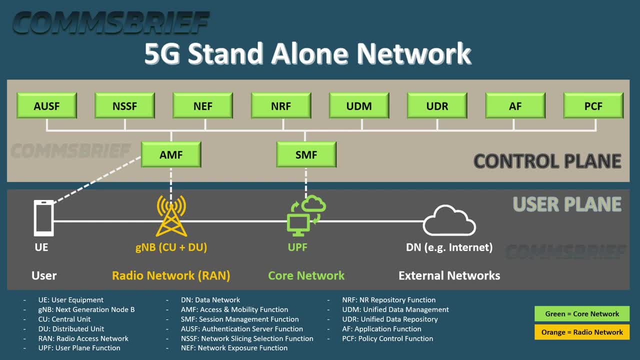 function SMF establishes and manages the sessions between a user device and the mobile network. It takes care of the management of IP addresses for the devices. It is also responsible for selecting UPF for the user device and for the mobile device. Finally, SMF is also an interface between the UPF and the policy control function PCF. 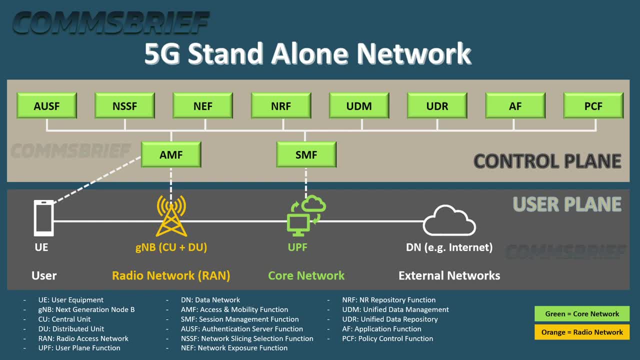 where policies and business rules reside. AMF, or access and mobility management function, is part of the control plane. It is connected to the GNodeB and provides access and authentication Network. slice selection function, NSSF, determines which AMF or AMFs the user can use to control the UPF.